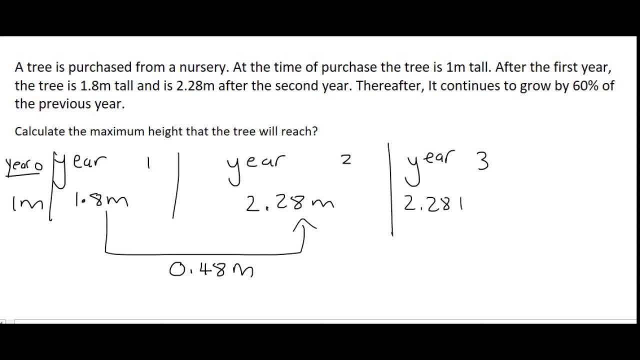 amount. so its new height will be 2.28 plus 60 percent, which is the same as 0.6 times the previous year's growth, which is 0.48. that is how trees grow. they grow fast in the beginning and then it becomes less and less each time. so the new height of the tree will be: 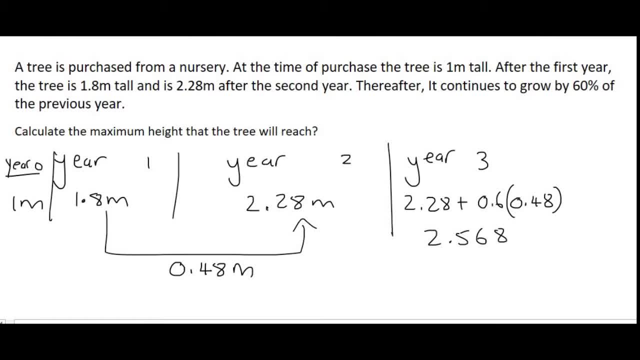 2.568. so just to save time, we can actually get away with, just we can stop right over there, we don't have to go all the way to year five. and so now we would have to try and form a pattern. well, to get from 1 to 1.8, well, there you would have to multiply by 1.8, or you could add 1.8. okay, so one. 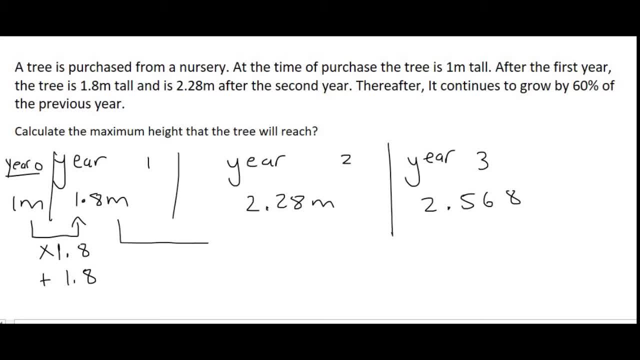 of those is going to have to work then to get from 1.8 to 2.28. well, how much would you have to multiply? well, that's difficult to see, but if we say 2.28, we can only get 1.18. okay, and so that? 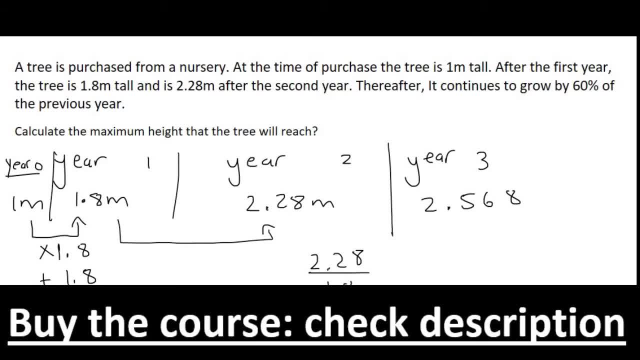 you just have to do is you just stop at year five, you just start at year three and then you start point two eight. divided by one point eight, that's going to give us a value of one point two seven. okay, so we have a bit of a problem, because now we're multiplying by one point two seven. 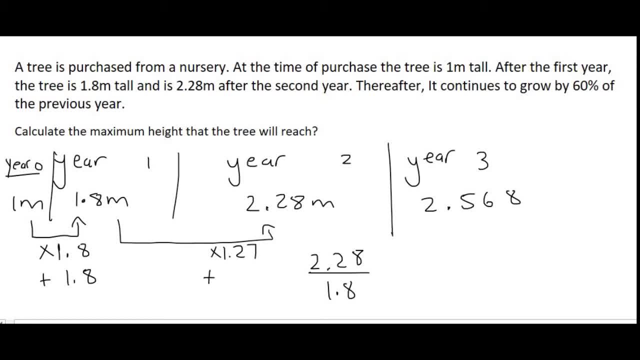 or you might be saying, wait, wait, we could just be plussing 0.48, okay, but now there's a bit of an issue because none of those numbers match what we did in the previous one. nonetheless, let's carry on. so to get from 2.28 to 2.568, well, you could say 2.568. to work out the ratio, you could say 2.568. 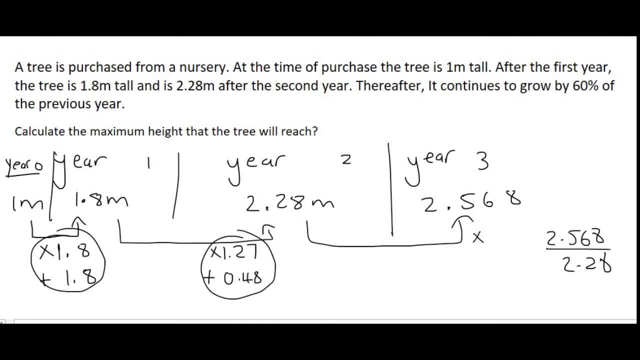 divided by 2.28, and that's going to be a ratio of 1.13, or we could realize. see how much we are adding, and that's 0.288. so what is going on? because nothing seems to be staying constant. we're not multiplying by the same number each time, we're not plussing by the same number each. 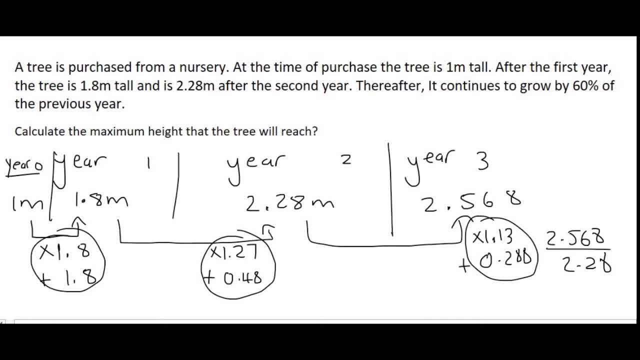 time we're not multiplying by the same number, each time we're not plussing by the same number, so there's no pattern. That would be correct. The pattern is not going to be formed by looking at the total height of the tree. The pattern is going to be formed by looking at how much the tree 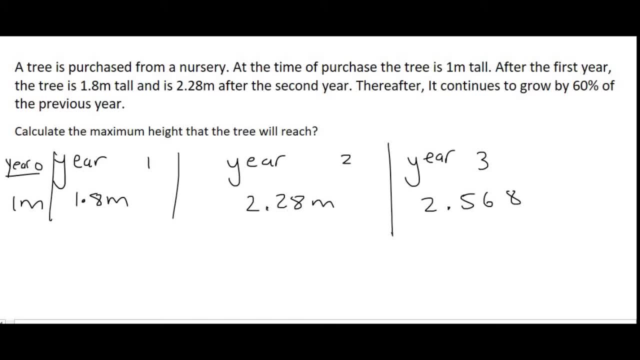 grew by each year. So we need to take a look at the growth. Okay, so in this, from year 0 to year 1, there was growth of 0.8 meters. Then from year 1 to year 2, that's 0.48.. And then from year 2 to 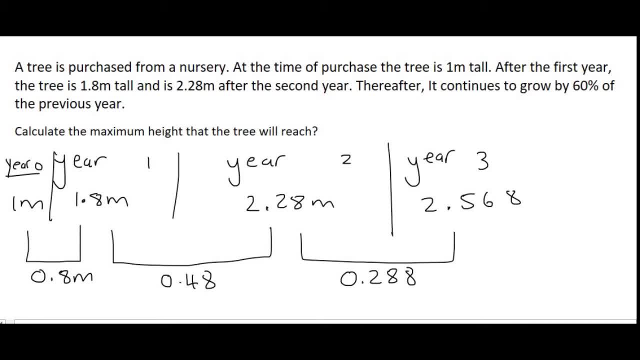 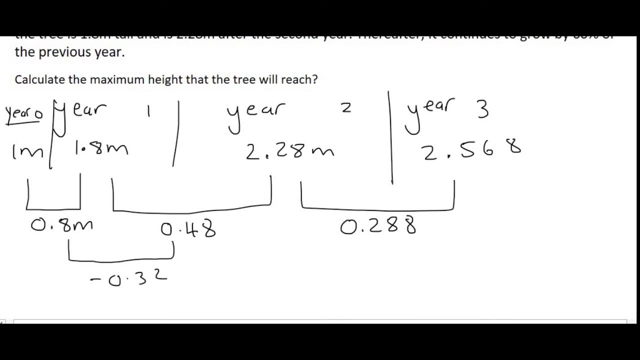 year 3, there is growth of 0.288.. So we could be forming an arithmetic or geometric. So let's take a look To get from 0.8 to 0.48,. we could be minusing by 0.32, or there might be a ratio. 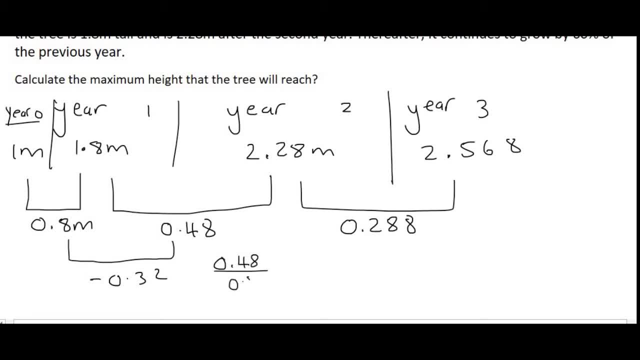 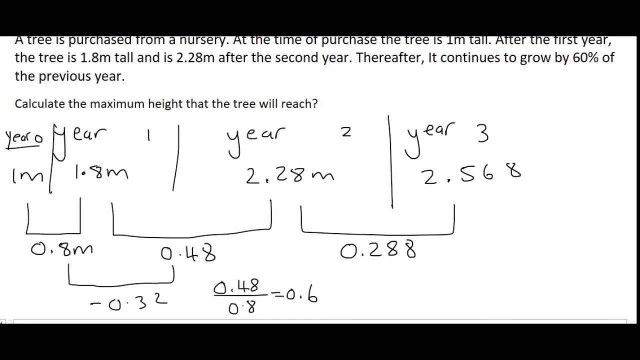 Now, the ratio is always the second term divided by the first term, and let's see what that gives us. And that's going to give us 0.6.. If we then look at the ratio for the next term, which is 0.288 divided by 0.488, it also gives us 0.6.. So there we have the ratio. The ratio is in the 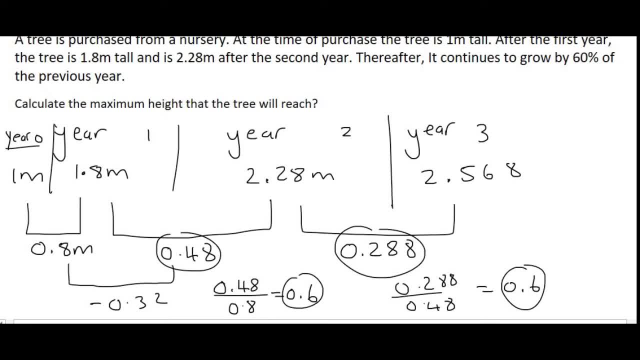 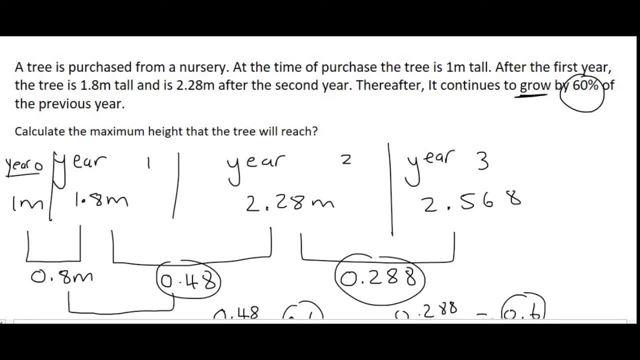 growth of the tree, not the total height of the tree, And that makes sense. They said that it continues to grow by 60% of the previous year. So because it's growing by a percentage of the previous year, that's going to form a geometric pattern where the ratio is 0.6.. So 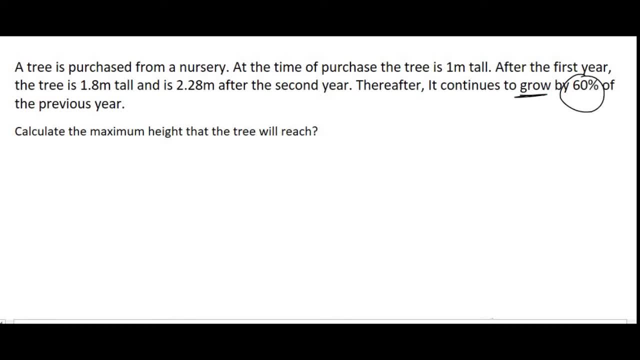 is the pattern with the total height of the tree or the growth. It's the growth, It's the amount that the tree grows by. So now they're telling us calculate the maximum height that the tree will reach. Well, now we have an issue, because we don't know how long the tree is going to grow. for 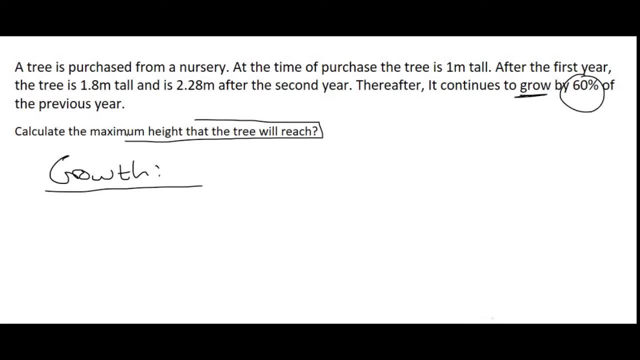 We don't know if we should do 20 years, 30 years, 40 years. However, if you remember our videos on convergent patterns, we said that if our ratio number is anywhere between minus 1 and 1, then we have a pattern that will converge and it will cause the sum to eventually stay constant. 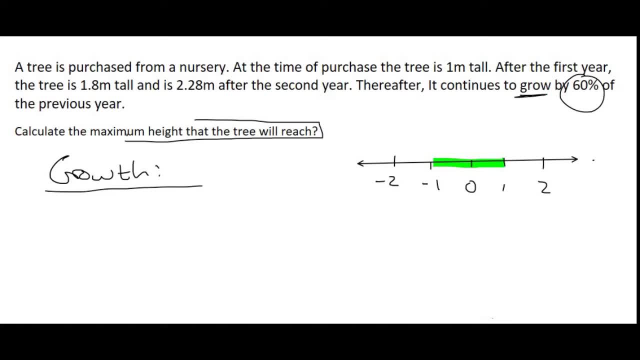 Now, what is the sum in this question? Well, remember the question that we did many videos ago, where we had a person who was saving money, but the amount that they were saving was becoming less and less. Well, in this question, the amount of growth is going to become less and less, And 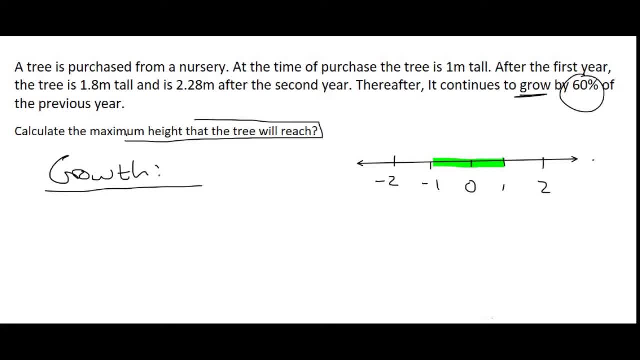 so the total height of the tree will eventually become constant. Just like in the question with the person saving money: their total savings eventually became constant. So we can use the sum to infinity formula. We are allowed to do that whenever they ask us to find the maximum and when it's a geometric 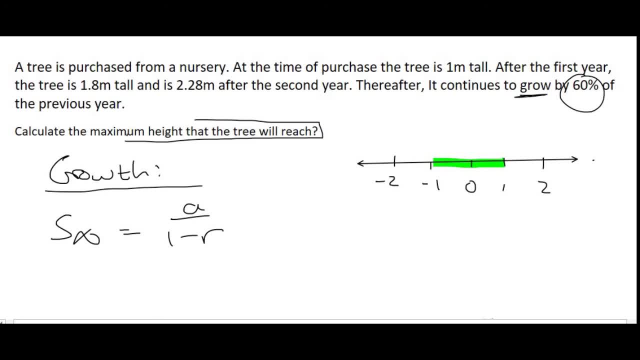 and it must be convergent. So R has to be between minus 1 and 1.. And our R is. we said that our R value is 0.6.. So we can use that formula. Now, what are we going to use for A? Now? this is: 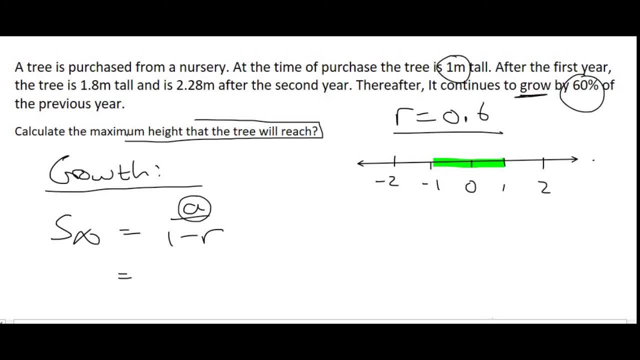 where we're going to use the formula for A. So we're going to use the formula for A. This is where many students will say: oh well, obviously it's 1 because that's the height of the tree. But remember, our pattern is not the total height of the tree, It's the growth And so the 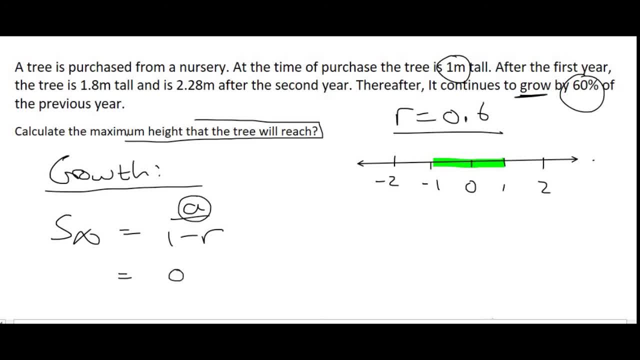 first growth that we had was 0.8 meters. It wasn't the 1 meter, It was the 0.8.. And even if we did use the 1 meter- I mean sometimes you could use the 1 meter, but check this out If it's 1 meter. 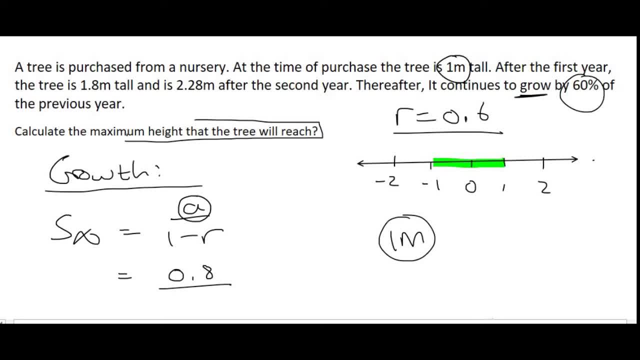 in the very beginning, after the first year, if we were to try grow the tree by 0.6,, that would only give us a total growth of 0.6 meters, And so the tree would have to be 1.6 meters at the end of the first year. However, they told us that the 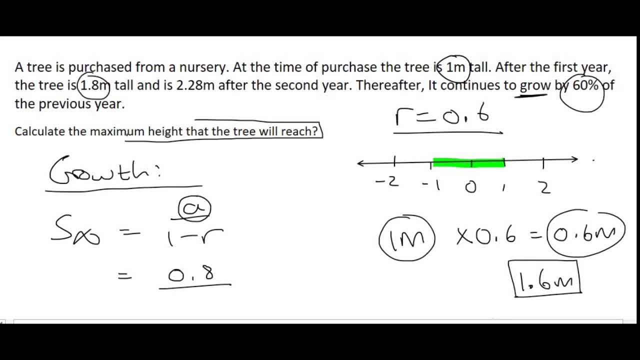 tree is 1.8 meters, And so the pattern doesn't work from the first year onward. Sometimes it will, but in this case it doesn't. That R value only starts working from year one onwards. So we're going to use 0.6 meters, And so the tree would have to be 1.6 meters at the end of the 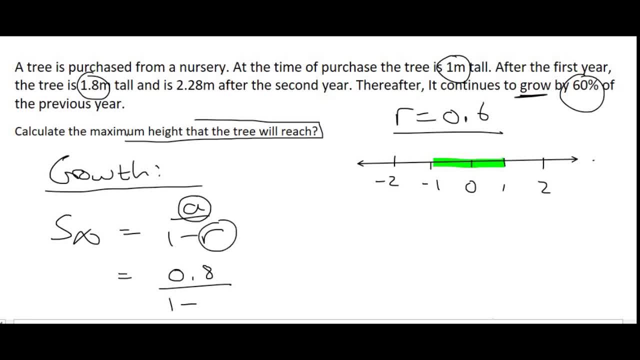 first year, But beginning from the first year, we might have to use 0.6 meters, And so the R value It's 0.8, a pretty simple right. We're going to use 1 minus once over three, so it should need to be. 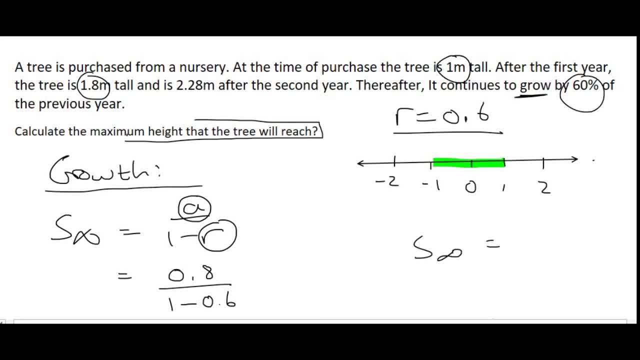 you'll see that we have to get one minus 1.8.. So we need to use another 0.8 over one minus, And the R value we're going to use is 0.6.. So you see, if we had used a as one, which is the initial height, 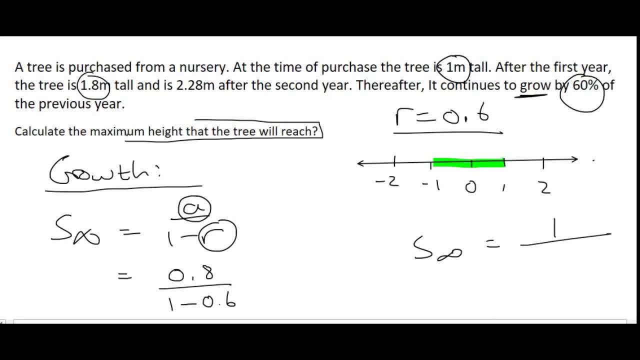 of the tree. that wouldn't make sense because the R value going from one to 1.8. That R value there is 0.8 and not 0.6. So we can't use the original height of the tree. we have to use, We can only- 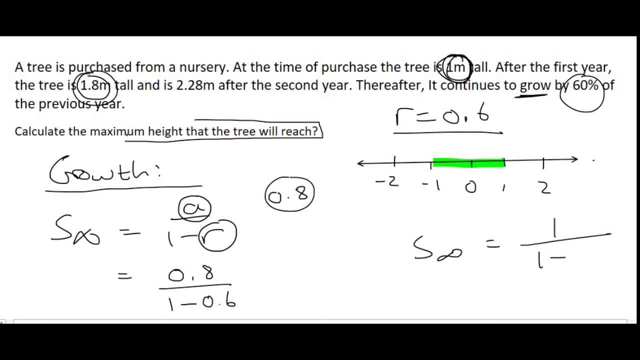 R values. there are 0.8, and that is not 0.6.. For 0.8, we have to reduce it to 3.5 meters if formula from the point when the r value was 0.6. i hope that makes sense. oh so no, we're not going to.